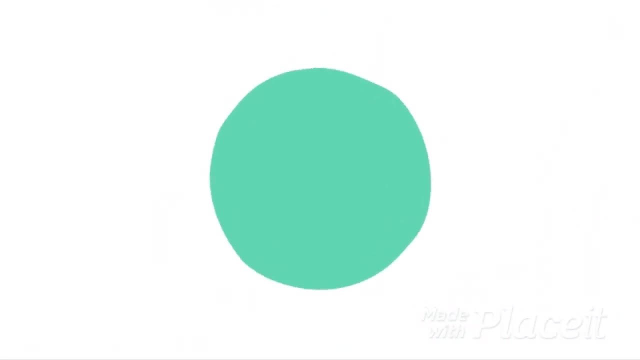 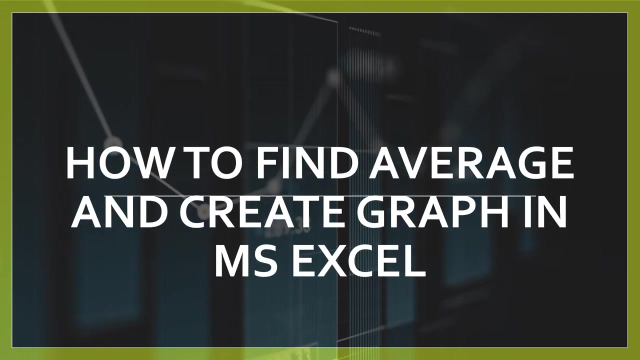 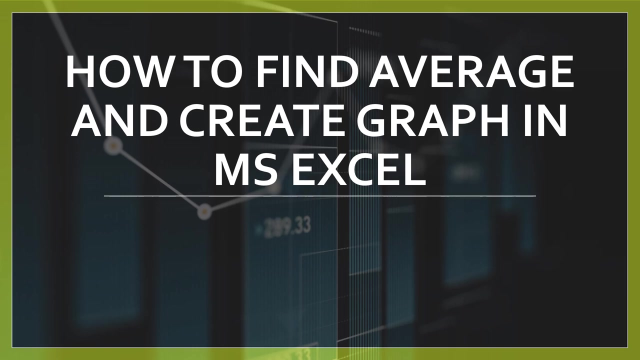 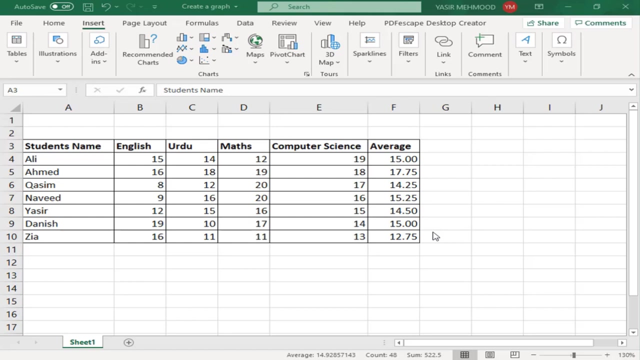 okay, friends, this is the practical representation of how you can insert a graph, and this video tutorial is a task number for task three. create a graph in this. first you will open the ms excel, and after opening the ms excel, then you will create a table like this: 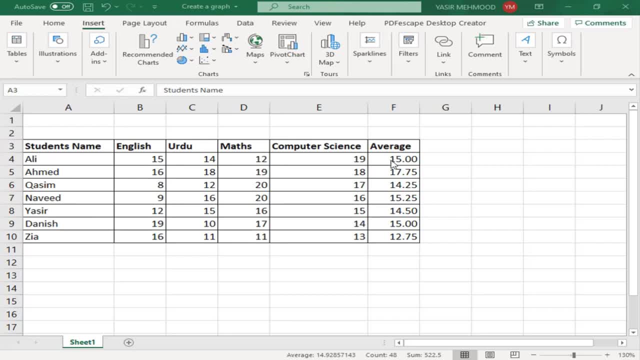 and you can enter marks and student name. this is the average. how you can find the average? you will write the formula for the average uh that you already studied in previous uh, previous task. so how you can insert graph. so, first of all, you will select the table. 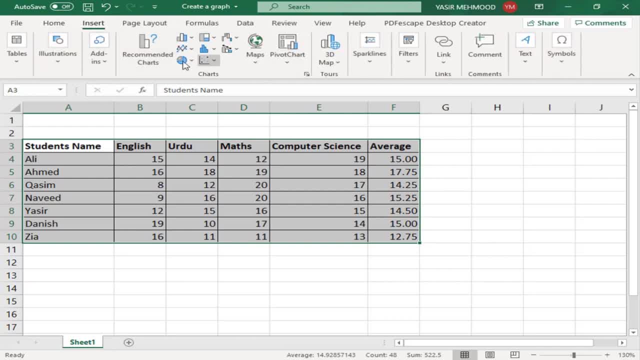 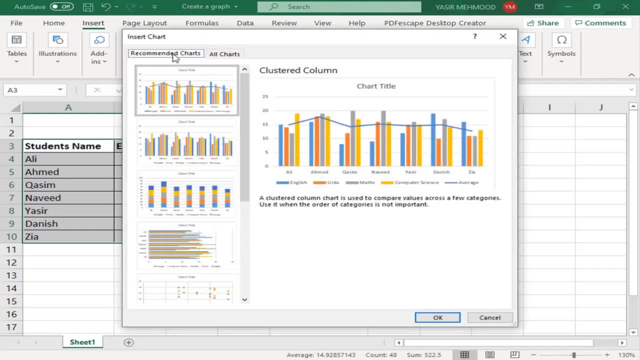 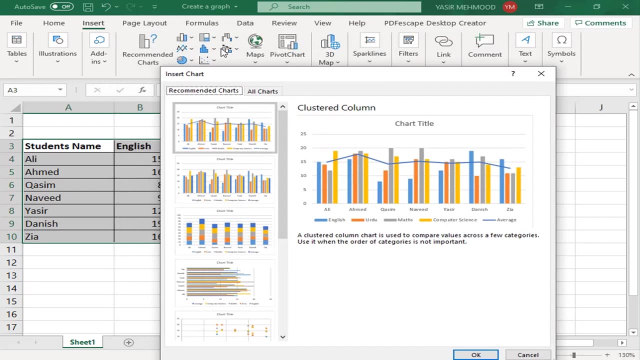 then you will go to the insert tab. there are a lot of uh charts are available, so you will click on this option up may expect. click on the head. then there is a recommended charts and all charts we're going to see here, like that. then there is an option there for the insert. 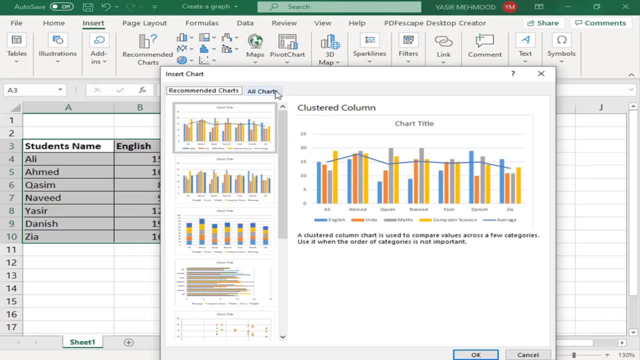 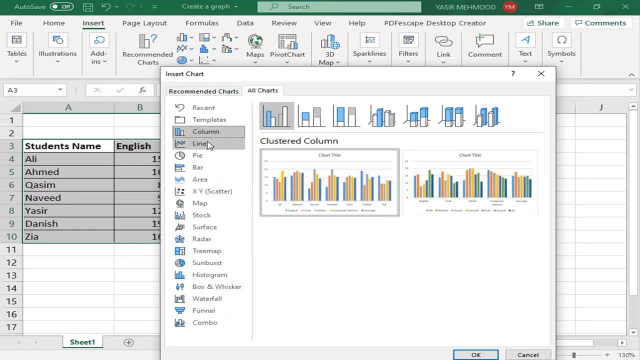 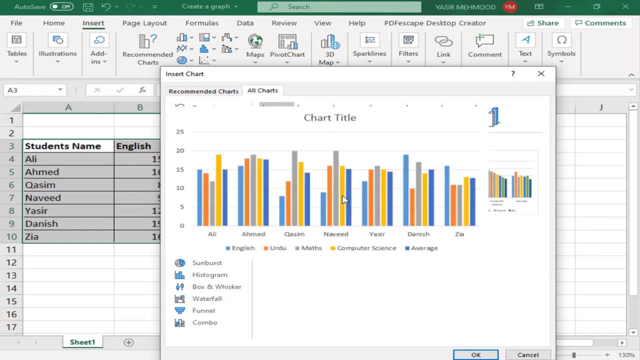 in the different type of all levels. so if you will select the one that is related to the other, then only the other. Pretty, this will be the old excel. so there will be a chart option in insert from which you will have to do it, but here is a little different. this is a little updated version. 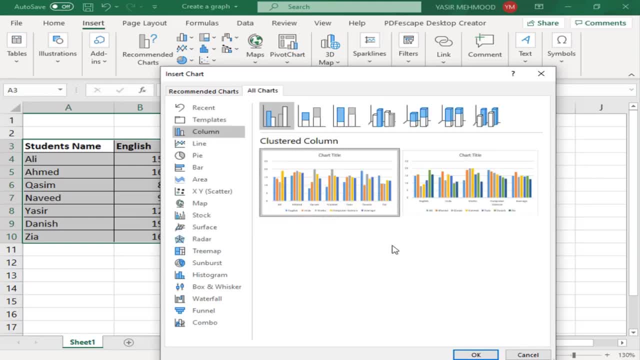 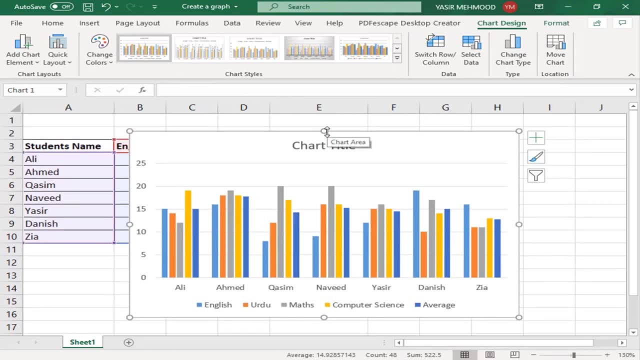 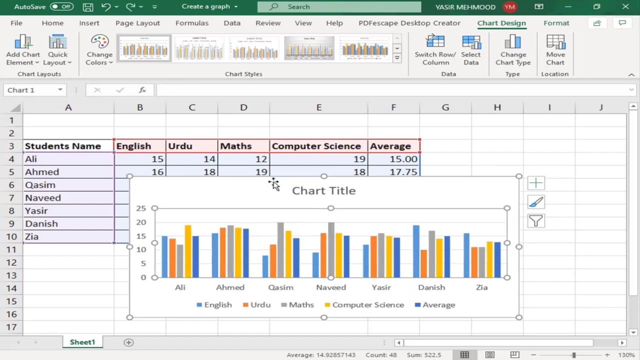 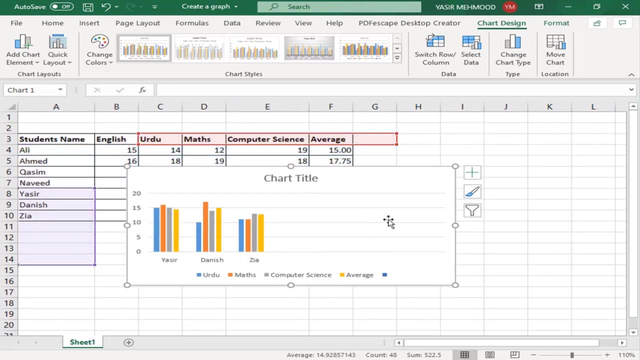 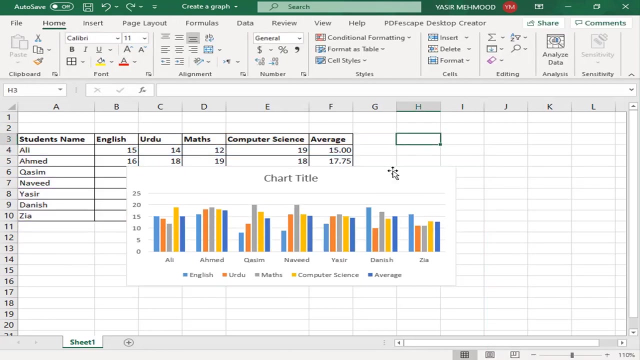 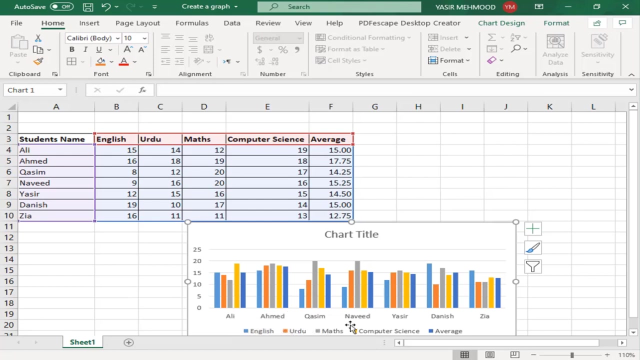 so you will click on all charts, you select this and click on ok. so this is the chart and you will move your chart to any location like drag. you can move it from here like this. so this is your chart: alice ahmed kasim n그�ید. yaasir danesh zaa.